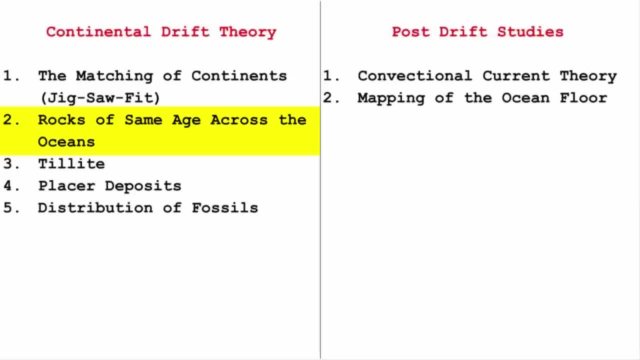 away Again. the reason behind the drifting is much deeper than just looking at rocks and saying they all are same. The third point in continental drift theory talks about tillite formation. The Gondwana land consists of six land masses. They are India, Africa. 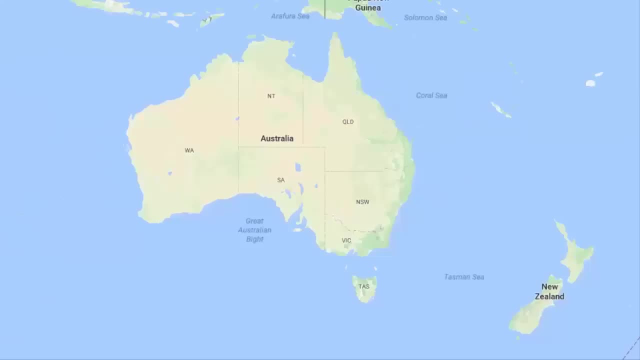 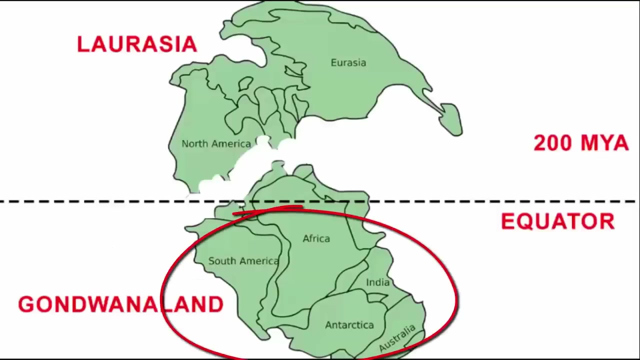 Madagascar, Australia, Antarctica and Falkland Islands. Under the base of these six land masses, tillite sediments were found, So that made Wegener think that, okay, these six land masses were once together and now they are apart. So this is a pretty good observation. however, the reason is: 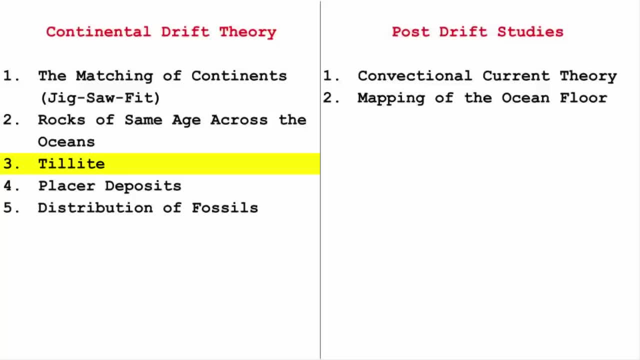 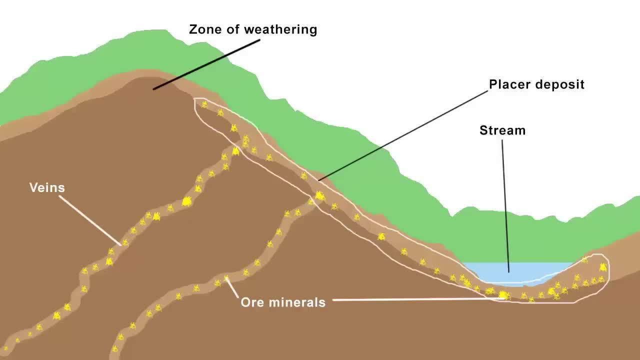 much bigger and in-depth rather than observing tillites. The fourth point in continental drift theory talks about placer deposits. They are deposits of rich minerals like gold, diamonds, etc. So if you look at the coast of Ghana and then coast of Brazil, you will see that these placer deposits looks like. 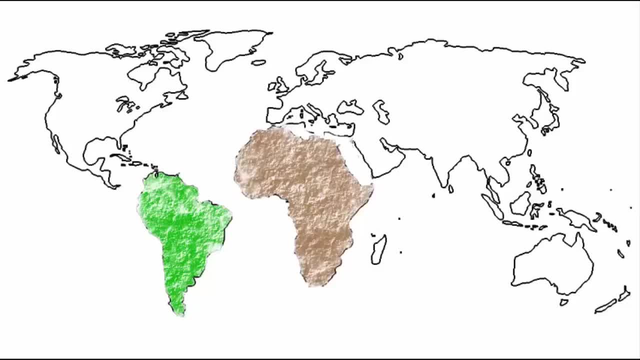 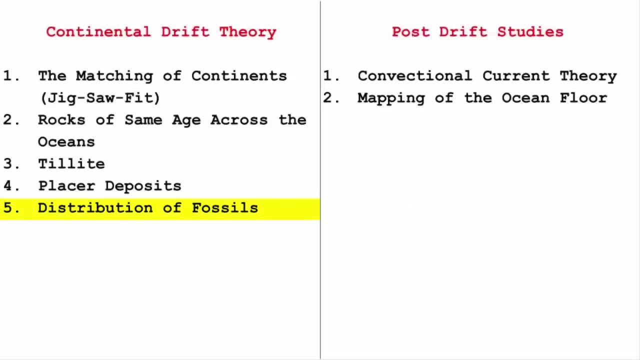 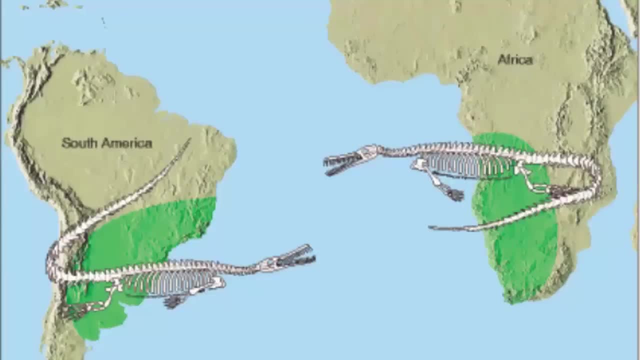 Wayne, that were once joined together. This point again made Wegener believe that Africa and South America was once a single land mass. And the last point in continental drift theory talks about distribution of fossils, When identical species of plants and animals were found on land masses. 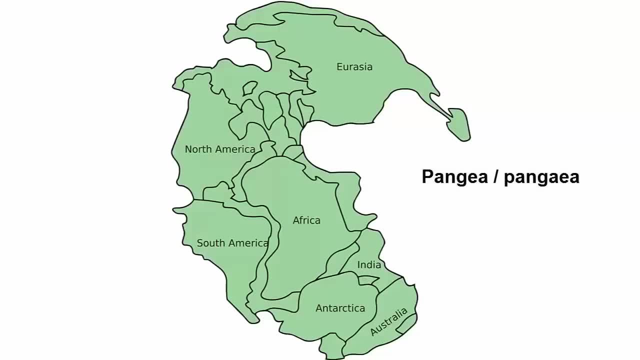 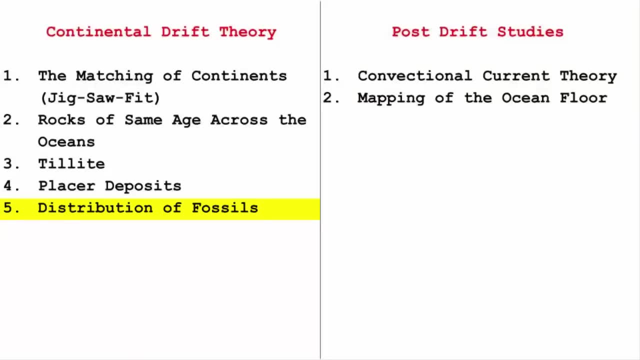 it made Wegener strongly believe that once upon a time there was only a single land mass, and with time it started splitting into different groups. So these were the evidences of Alfred Wegener that made him come up with the continental drift theory. Now coming to the right hand side, that is the post. 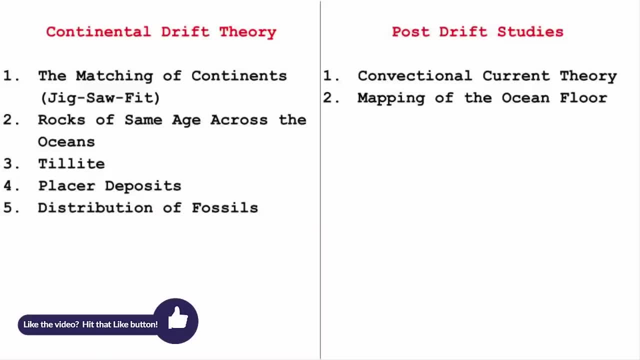 drift studies. After the World War II, many discoveries were made which added new information. Scientists started arguing the fact that Alfred Wegener only looked at evidences that were collected from the continental areas, Which is true If you look at the left hand side. 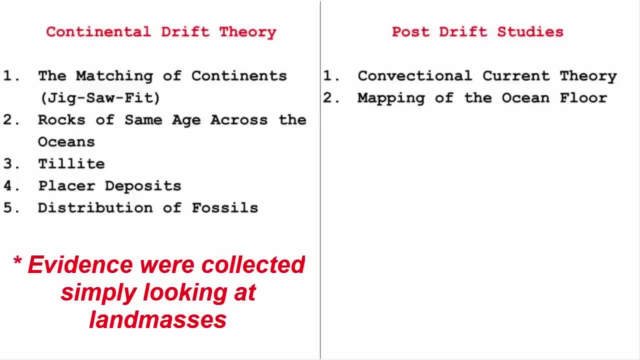 all these evidences were taken by simply looking at the land masses. So in the post drift study the scientists felt, hey, why don't we do some comprehensive study by mapping the ocean floor? and that led to the convectional current theory where Arthur Holmes said it is because of the 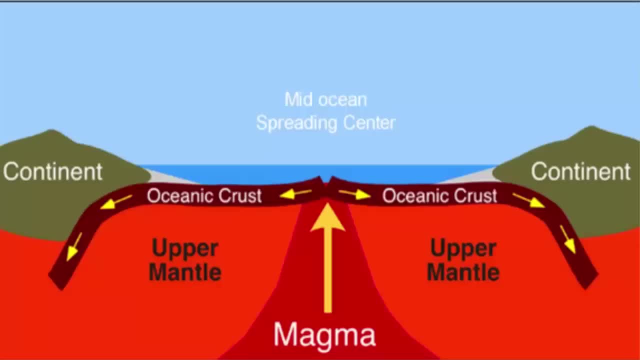 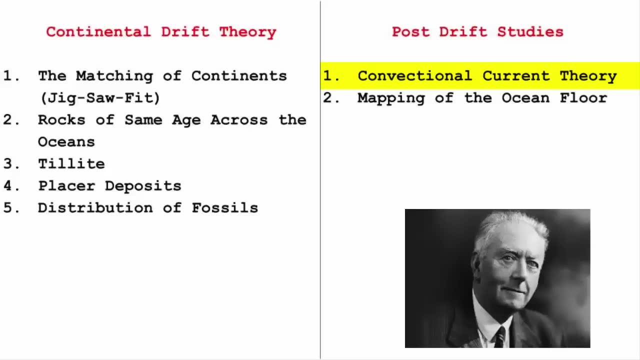 magma present in the mantle, which is causing the ocean floor to expand, Since the oceanic crust is thinner than the continental crust, therefore, it is easy for the magma to come out from the ocean bed, and that's why the mid-oceanic ridges give a solid proof about this theory. And the second: 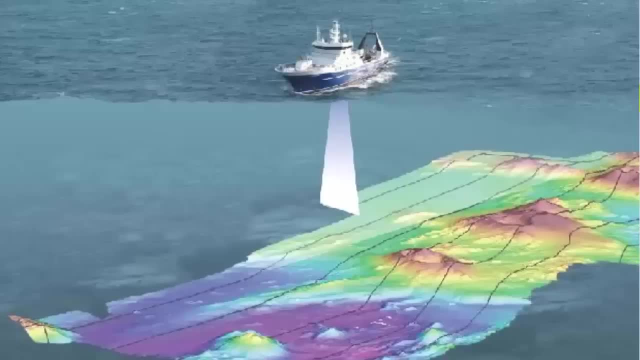 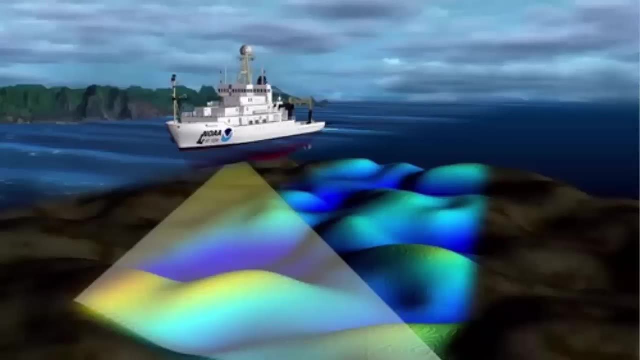 point in post-drift theory is the mapping of ocean floor. When the ocean floor was being mapped, scientists saw that ocean bed is not a flat piece of land. It has similar terrain, uneven surface, just like we have on land. This was an astonishing finding, and then they also went on to find: 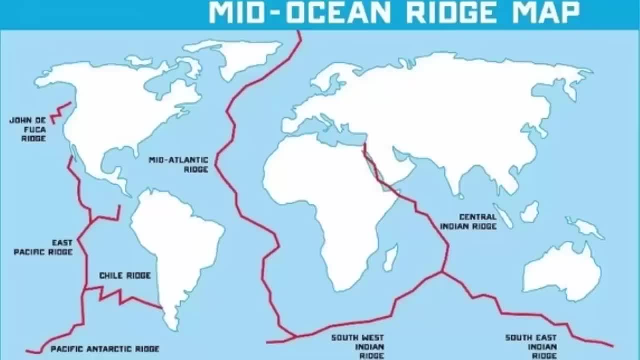 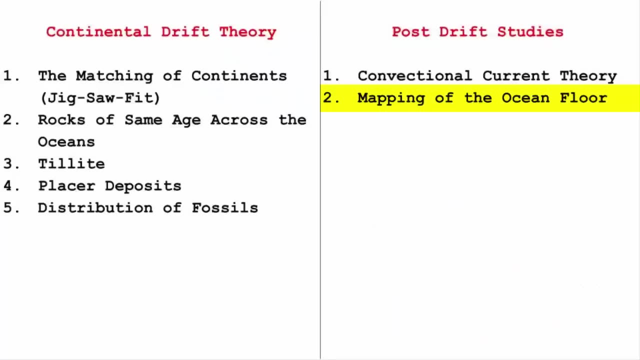 mid-oceanic ridges on the ocean bed, which are these long range of mountains that were formed due to the rocks that came out of the mantle in the form of magma, And when scientists took samples of rock from the mid-oceanic ridges. 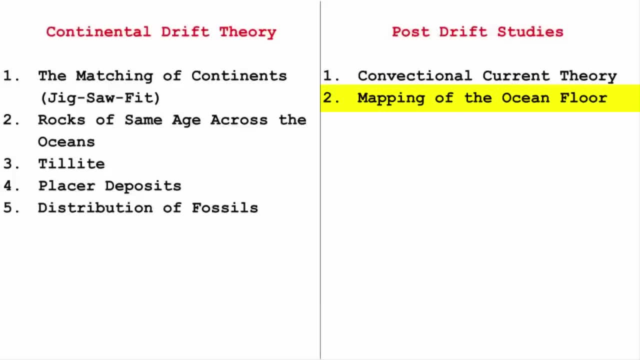 as well as from the continental side. they found that the rocks from the mid-oceanic ridge were comparatively younger in age. Hence, they concluded, as we move away from the mid-oceanic ridges, the age of the rocks increases. So this was the post-drift studies, which totally focused. 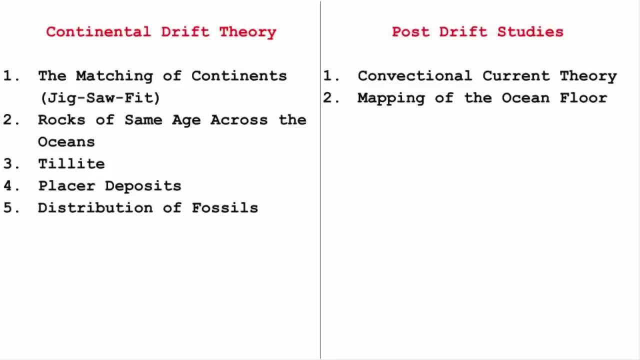 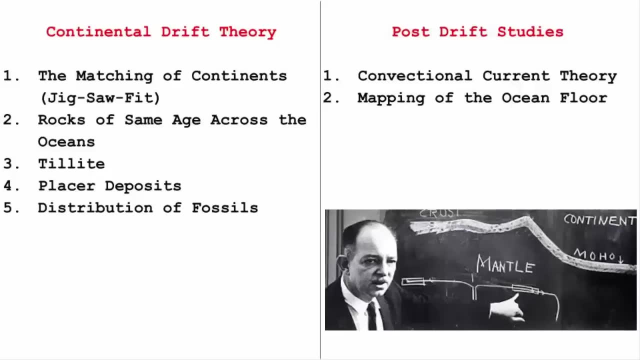 on the concept of sea floor spreading, That is, the ocean floor gets pushed to the opposite side due to volcanic eruptions at the crust and making the sea floor spread, and it was presented by Harry Hess in 1961.. Whereas the continental drift theory by Alfred Wegener focused on the argument that all the 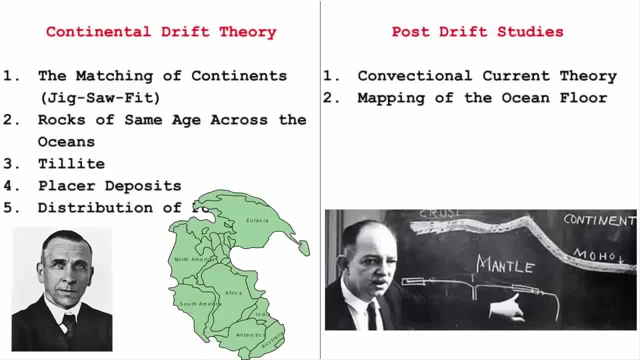 continents were once upon a time a single continental mass named Pangea, And then this single continental mass began to split into smaller ones, and that's how the world looks today. Hold on, we are not done yet. Now we have a third concept, which brings us to the topic. 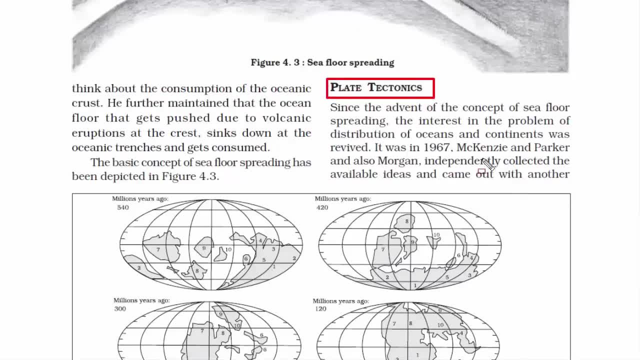 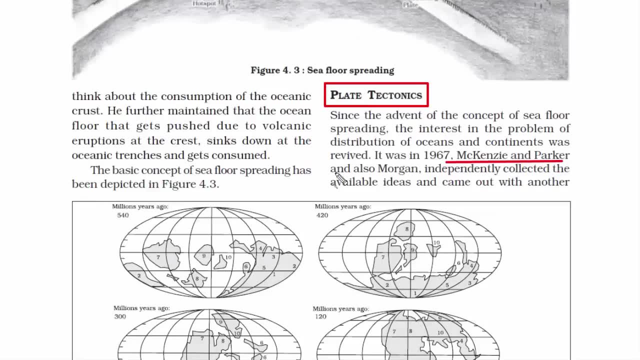 plate tectonics. Now this is the third concept that tries to answer the questions related to distribution of oceans and continents. Plate tectonics was presented by McKinsey, Parker and Morgan- 3 people- in 1967. Just after 6 years of Hess's sea floor spreading theory. So what plate tectonic concepts say? 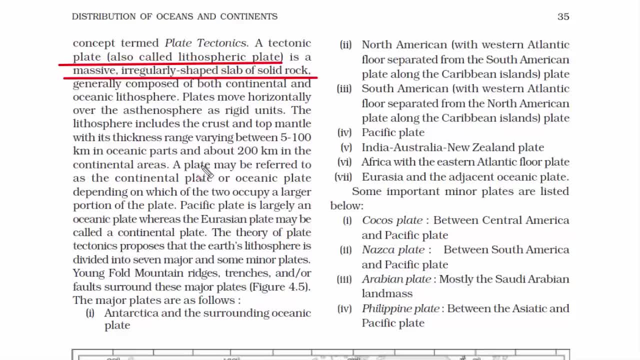 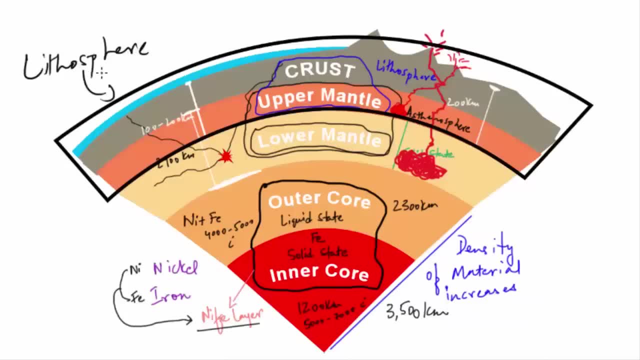 is the lithosphere- which is also the combination of crust and upper mantle- is in the form of irregular slab of solid rock. So think of the lithosphere as a large plate, and now, when a plate breaks, this is exactly what it looks like When we say irregular. 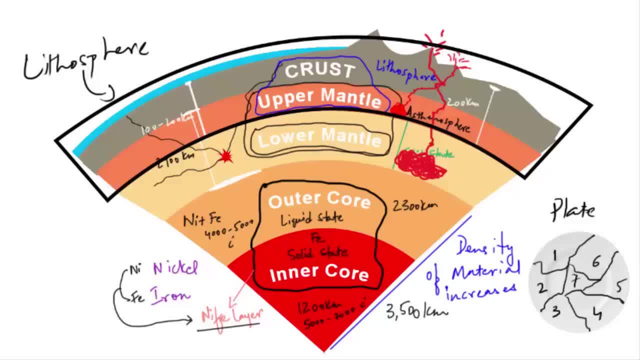 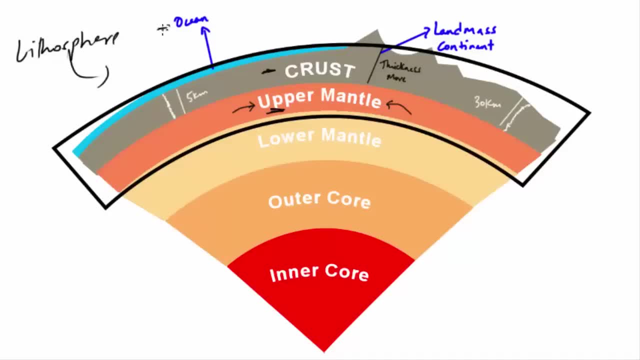 slab of solid rock. this is what the plate tectonics concept is suggesting. So we know that lithosphere consists of crust and upper mantle, And the crust is both continental as well as oceanic in nature. The oceanic crust is thinner than continental, but in